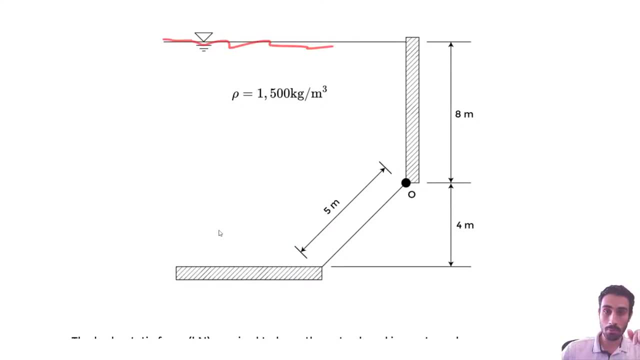 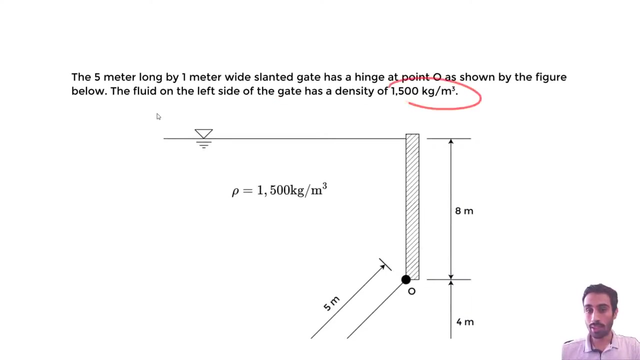 have is a gate down here that is submerged below a top water surface and its 5 meters long and the width into the page is 1 meter And we have a hinge at O in this particular case And we are told the fluid on the left side of the gate has a density of 1500 kilogram. 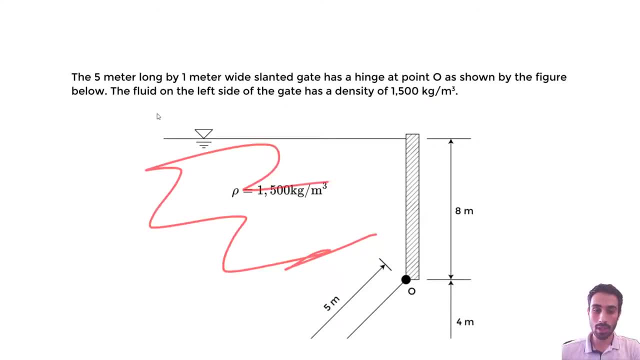 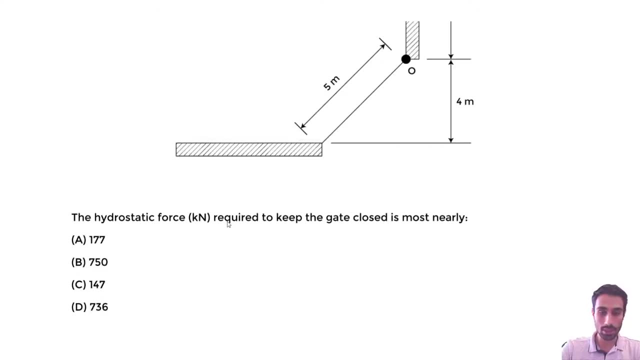 per meter to the third. So this is the density for the fluid on this side And, based on this case, we want to look at the hydrostatic force in kilonewtons. Kilonewtons required to keep the gate closed is most nearly what. So we know this side. 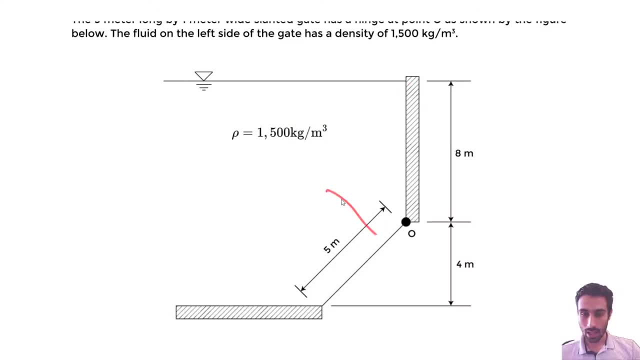 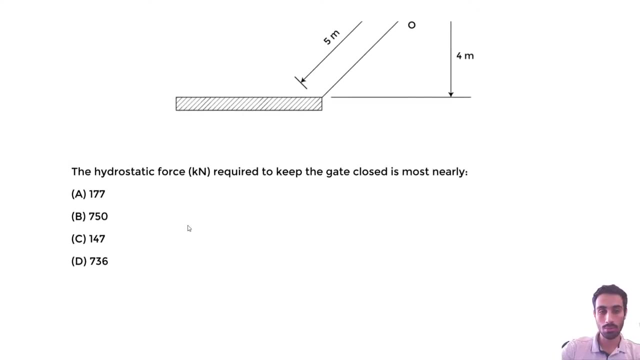 will have the fluid. It has this density and the fluid always distributes some pressure. So we have a distribution of pressure and what we want to find is the force. So we want to relate that pressure to a force And that is what we are finding here in kilonewtons. 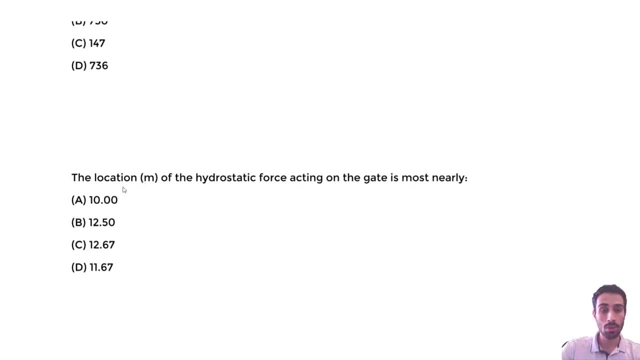 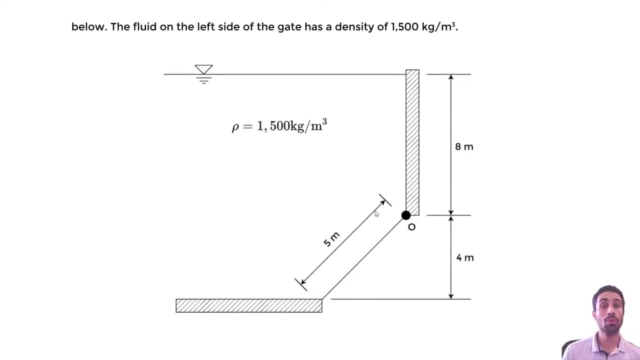 The hydrostatic force due to the fluid And at the bottom we will also solve this and find the location, The location of this force for that slanted gate. So the first thing I recommend we do is draw the pressure distribution And we know in the handbook this is also provided. 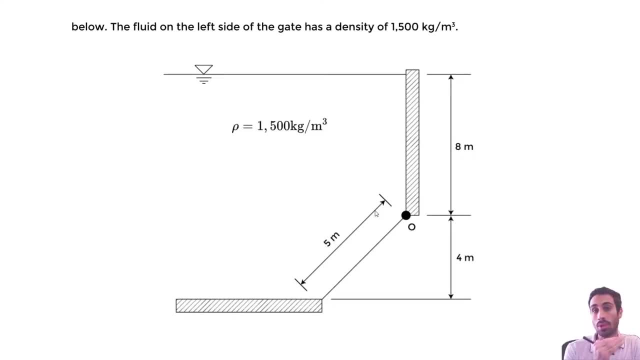 in the new FE handbook. They drew the pressure distribution for us and from this pressure distribution we can find the force. So let's draw this pressure distribution And it would look something like this: We know the pressure is always perpendicular to the surface. we 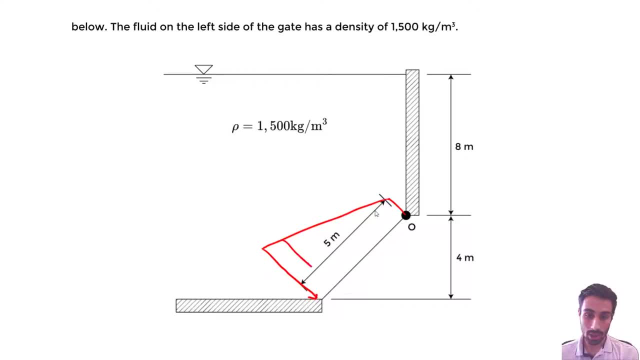 are looking at, And in this case it is the gate. So this is our pressure distribution. So from this pressure distribution we want to find a resultant force- And I will use blue for that- And let's say it acts somewhere here. This is what we want to find: The hydrostatic. 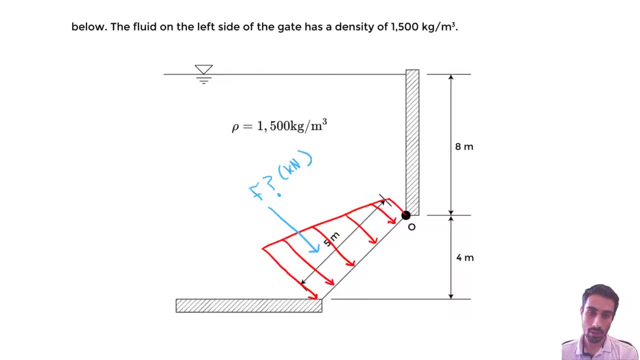 resultant force in units of kilonewtons. So based on that, we know that we can develop two basic shapes if we choose to. But that's the more complicated part, The approach. So that approach is more complicated when you are looking at these slanted gates. 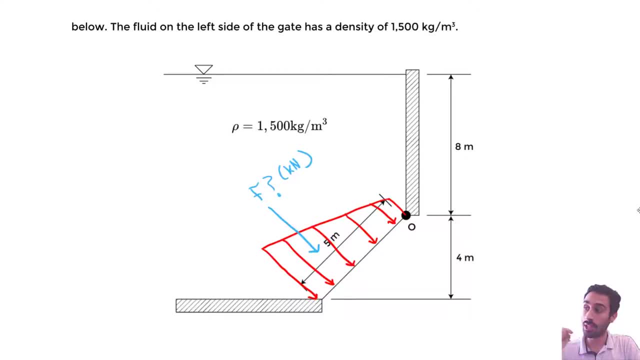 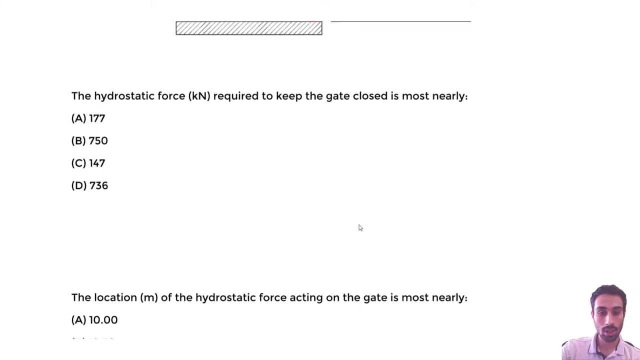 So what I recommend for the FE is make use of the equations in the handbook. So it's under fluid mechanics, It's under the forces on submerged surfaces and center of pressure. The major equation you have to know is the hydrostatic resultant force equation. So let's 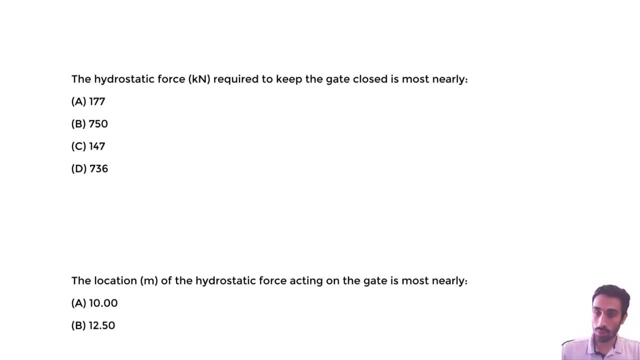 write that down. So the hydrostatic resultant force equation, which is what we want to find. It's under fluid mechanics. So what I recommend for the FE is make use of the equations in units of kilonewtons. So let's write that down. So what we have here is the hydrostatic resultant force equation. 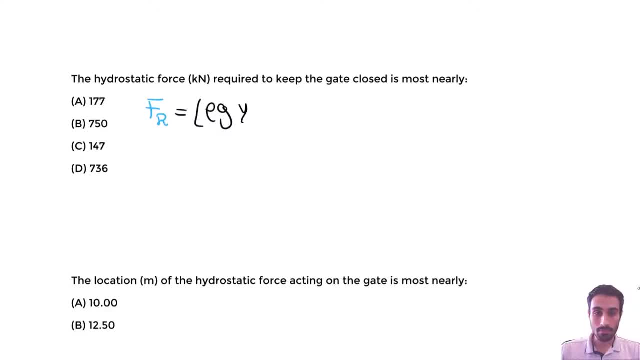 And then we have our heat transfer. So what we do is we take the density and the density of the area, And we take the density and the density of the area And then we do the sine of theta And all of this times the area. So we know that. Let's look at what we have. 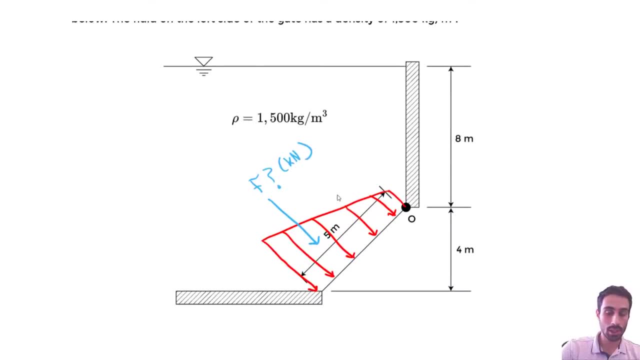 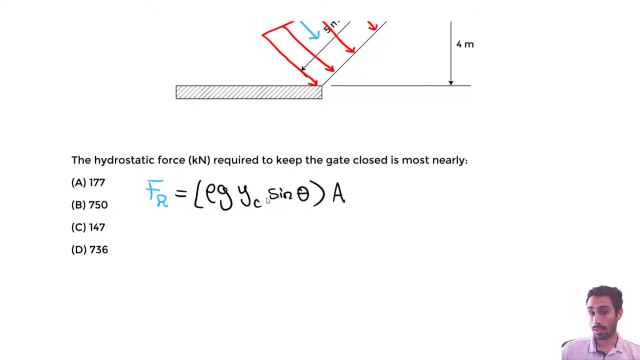 and what we don't have. density right, That's 1,500.. We know G is 9.81 in SI YC. we do not know. We do not know theta and we know the area. We know the area because it's just the five meter by the one meter wide. 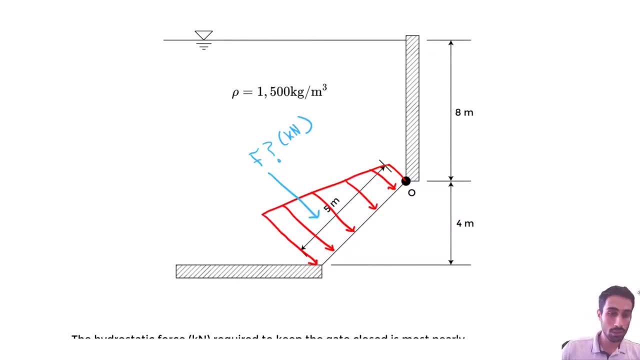 gate. So we're looking at it in 3D, So we're looking at it into the page. So let's say: this is our gate, We want to look at it into the page and we're considering this gate right. 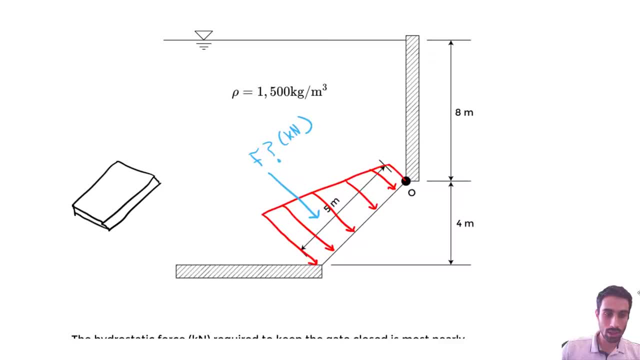 We have something that looks like this, and we know this distance is essentially like the height. right, It's the length, which is the height if we look at it from that view. So it's going to be the five meters, and this distance, where we are told into the page, is one meter wide. It's. 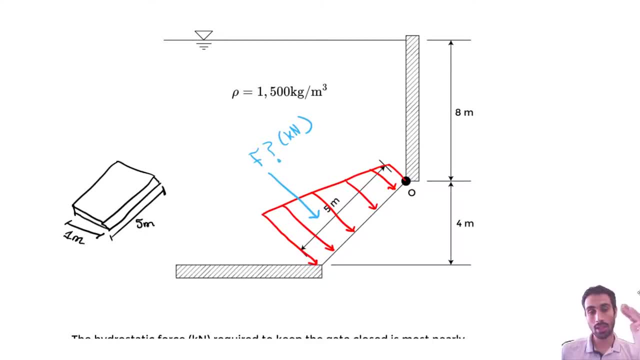 essentially the base. So you want to look at it in that view when you're doing the area. So the area is the cross-sectional area and we know that's where the gate is. So we're looking at it in 3D. 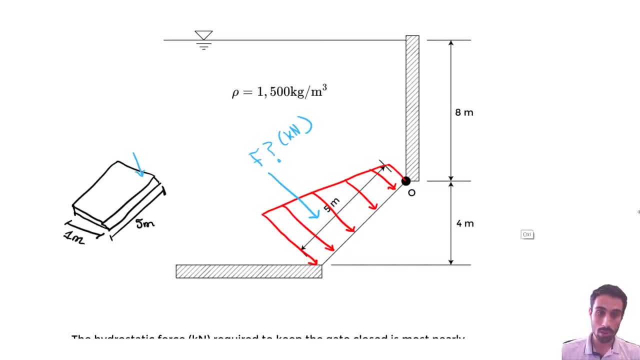 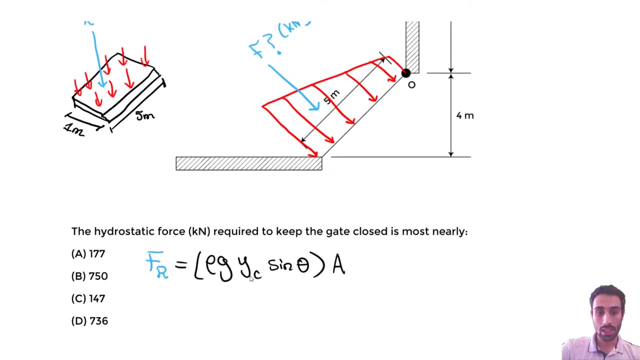 The pressure is going to act, the pressure distribution. right, Let me use red as I denote it in the figure. So that's what we have. This is the pressure distribution, and what we want to do is find the resulting force, FR. So that's just the 3D view of that gate, the slanted gate. So we know we need YC and theta. 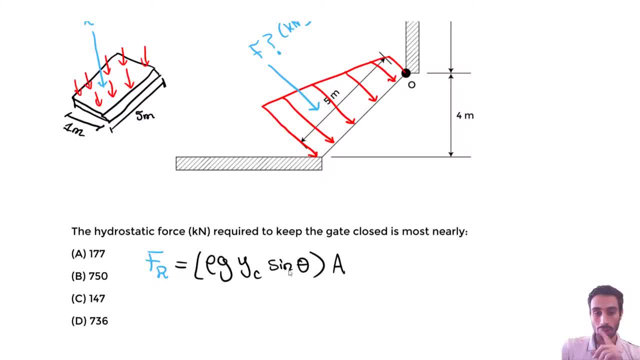 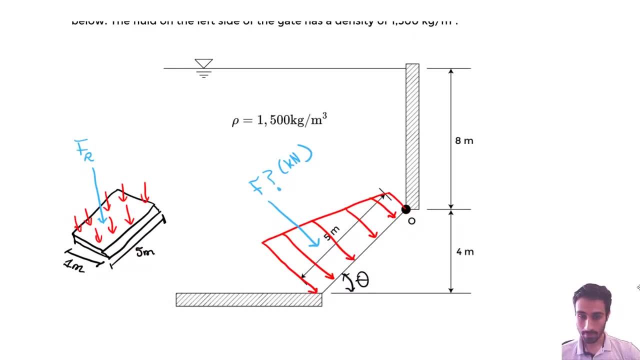 The area we can find is just five by one, right? So let's find theta real quick. So theta is going to be this angle, right? So it's that angle and that's what's denoted in the figure in the handbook. They denote the angle here. 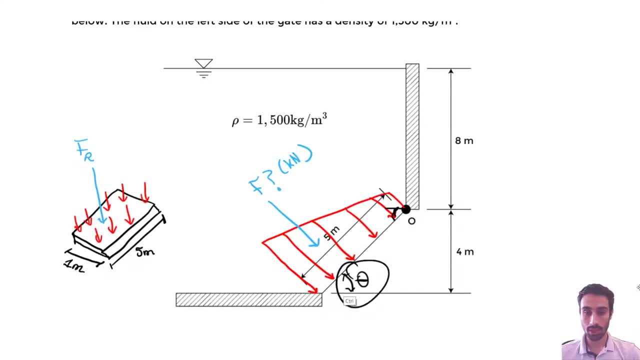 so it's similar to this angle. We know this angle is the same as this angle, So that's your theta always. It's the angle with respect to the horizontal up to the slanted gate. This is the horizontal and we move this angle to the slanted gate, Or, if you look at it from: 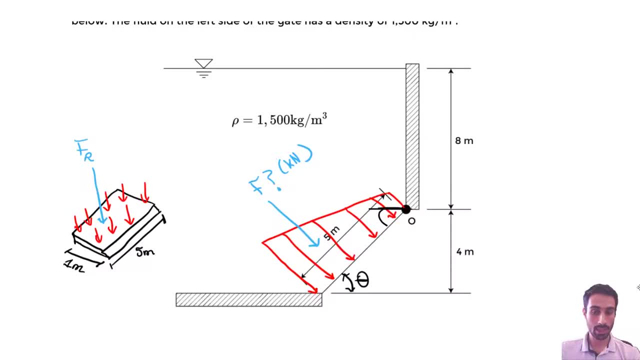 this view, this is the horizontal. We move this way, at this angle, to the slanted gate. So that's theta. and we can find theta by doing what rule? So we know, SOHCAHTOA, Which one can we use? So, because we have the opposite and we have the hypotenuse right, So we do. 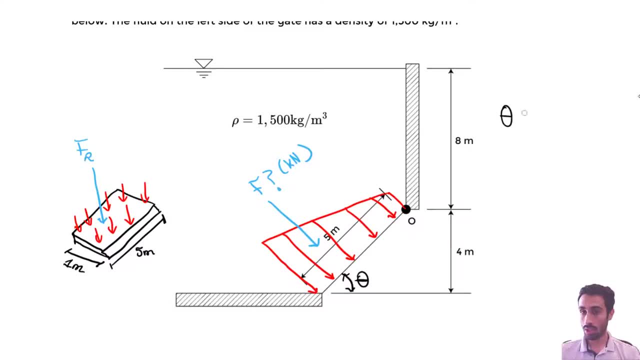 the SOHCAHTOA which says: let me denote that. It says: sine of theta equals the opposite over hypotenuse. We do: sine of theta, What's the opposite? It is four meters right. The opposite is this side, so it's four meters. The hypotenuse is this, so it's five meters And you can. 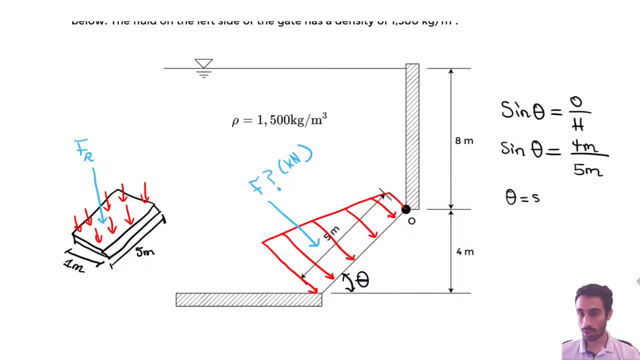 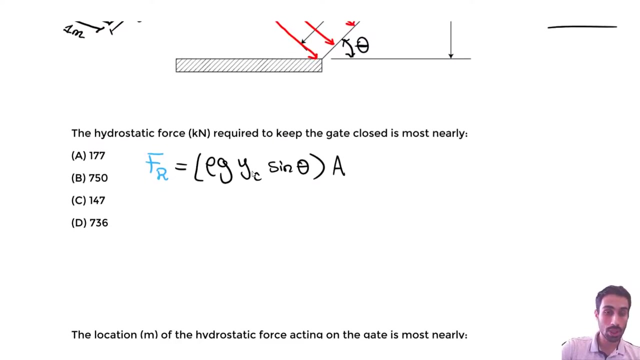 do sine inverse now. so theta equals sine inverse in the calculator of four meters over five meters. So we can find theta and I believe you should get. let's see 53.13. Degrees. So we have the angle theta. We need that in order to plug it in this equation. 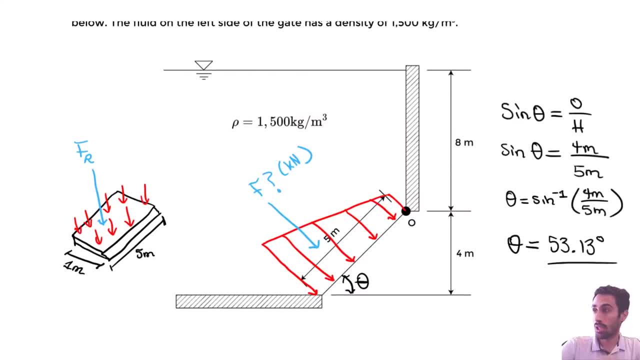 Now let's find YC. So YC is the tricky part. So Y, always for slanted surfaces, is from the very top water surface and it will be a slanted angle. It's not a vertical, it's not a vertical distance, It's a slanted distance. 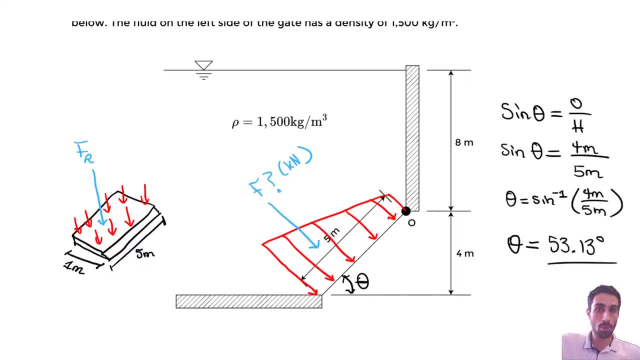 So it's going to be parallel. So it's going to be parallel. So it's going to be parallel to the gate. Always remember: Y is parallel to the gate. So we know. in this particular case, let's say: I draw this line all the way to the top. 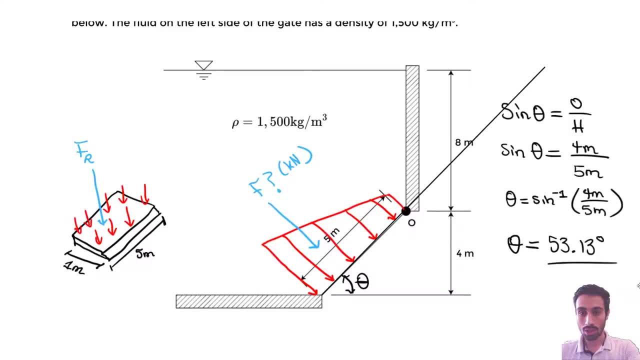 surface right. I want to match the top surface, So that's my line here. So this is the top surface right. We always start at the top, at the top. So Y is going to be the distance YC is going to be from that distance to the centroid. 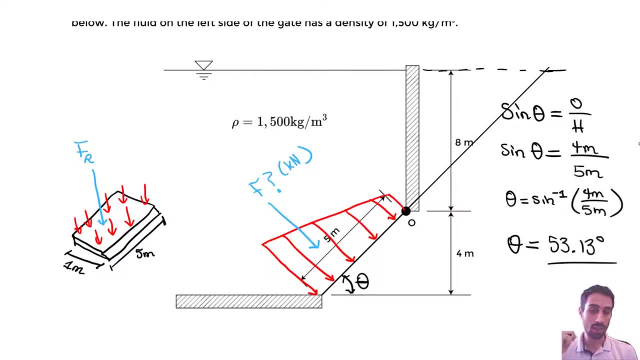 The centroid of the gate, So the dead center of the gate. The centroid of the gate is just at the center right. So in the last slanted gate example that I uploaded the top surface was just here right. It made it easier. But here our top water surface is at the very top, So we have to 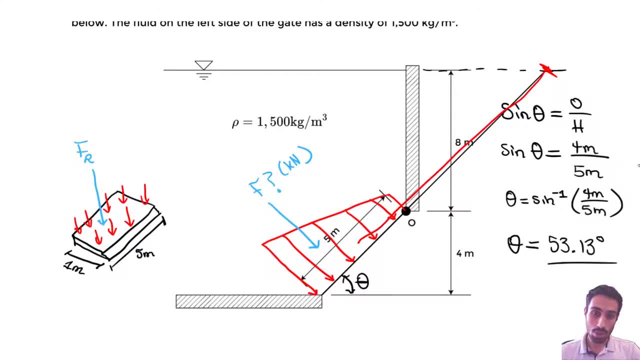 account for this entire distance from the top to the centroid. So we know here I'll denote it by this color- actually green YC is going to go to the centroid of the gate. So the centroid is somewhere here of the gate And we start at the very top and go. 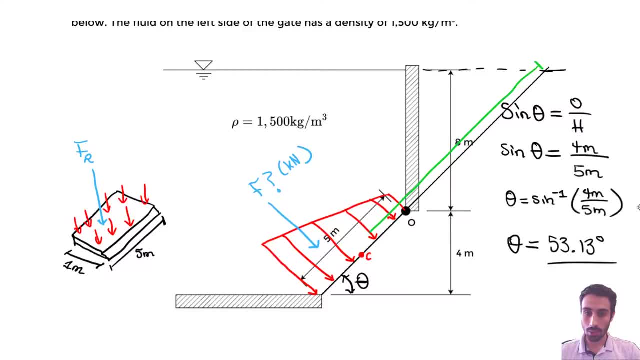 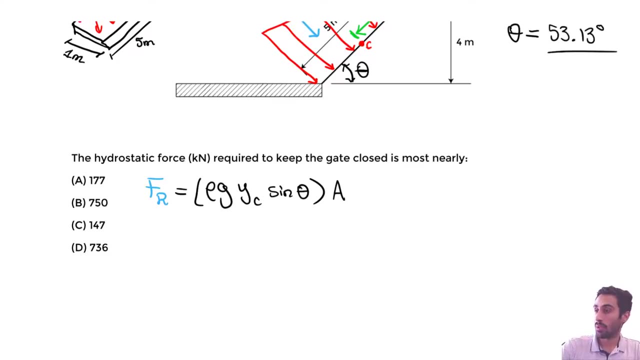 all the way to the centroid And that's what we need to find, That's what we're finding and that's going to be our YC. So that's what we need to find in order to finally solve this equation. But we know in the handbook it makes it easy for us. They just give us the equation. 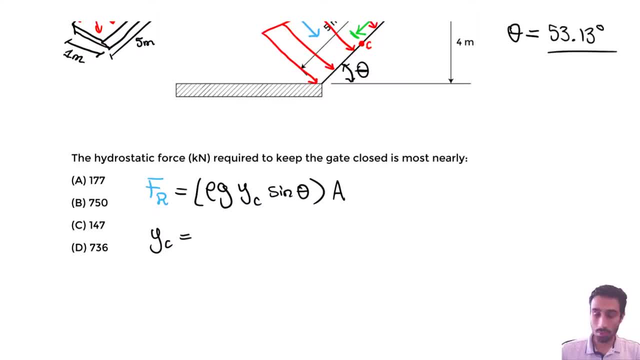 So YC is going to be HC divided by sine of theta And we know theta right. We just found that, So we can easily solve for YC. And let me denote that with green That's the YC we want to solve for And plug it in here. We just take HC divided by sine theta And we 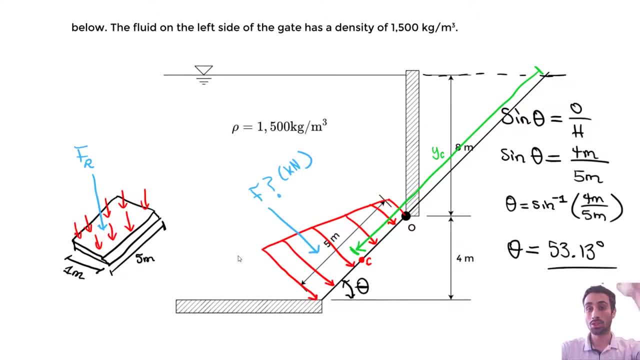 know HC is always vertical. It's strictly vertical from the top water surface. So what we have to do for HC is start at the top and go strictly vertically downwards to the centroid. That's what we denote by C. This is HC. So we know HC can be easily found right. We just take the 8 and take the 4 divided. 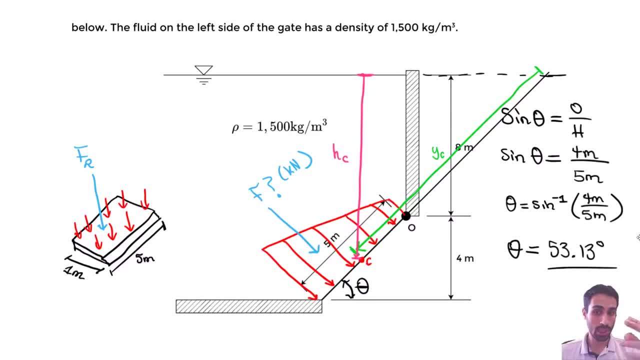 by 2.. 4 divided by 2 is 2.. We take 8 plus 2.. Once again, we take this distance, which is 8, right. Then we add this distance to the centroid, which is 4 divided by 2, right. So the total HC is: 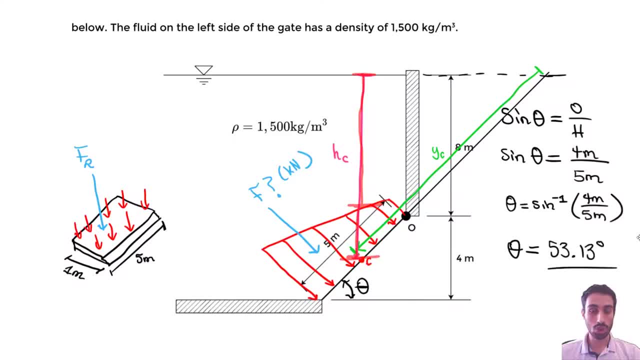 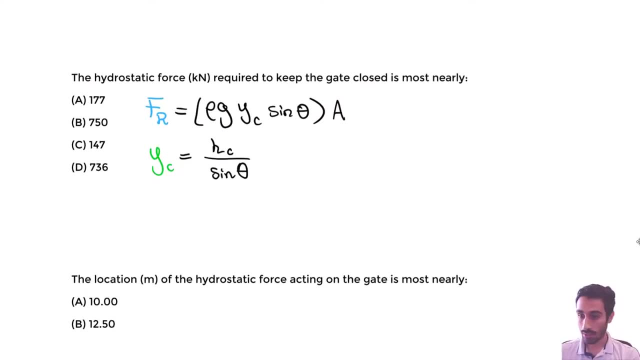 8, this distance plus this distance, which is 4, divided by 2, which is 2 meters. So HC is 10 meters. So let's denote that We can say in the equation: We take the 8 meters plus 4 meters divided by 2.. Then we do sine of theta And we know: 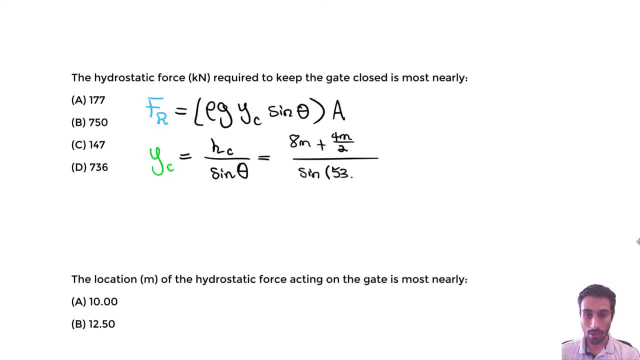 theta is 53.13 degrees, So now we can solve for YC And you should get 12.5 meters. So we just found YC Basically. what they did is trick. They found the YC Basically. what they did is trick. They found the YC Basically. what they did is trick. They found the YC. 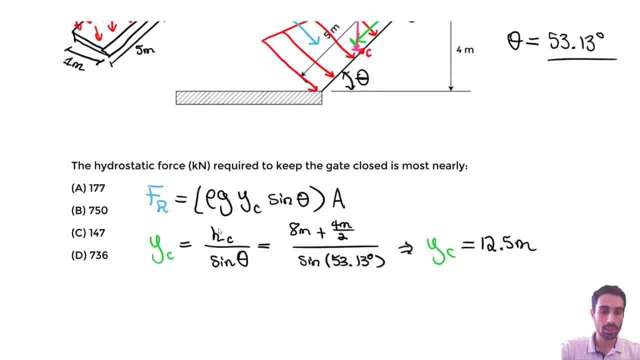 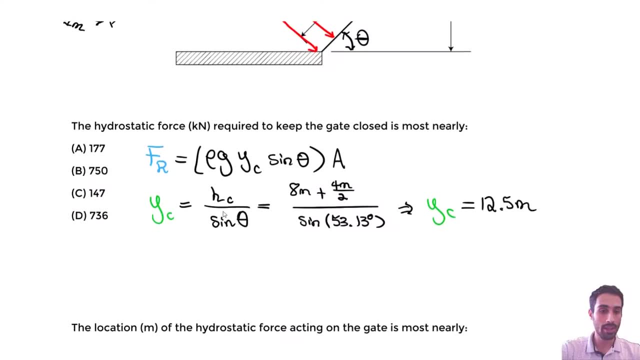 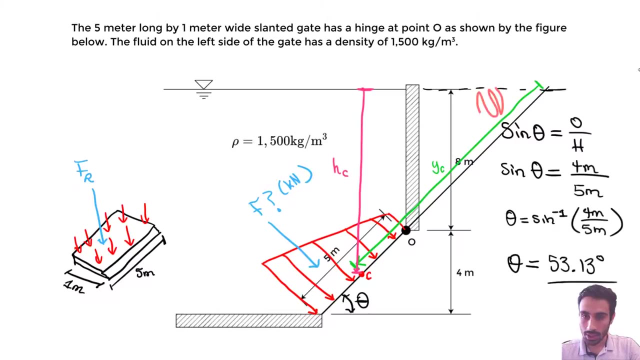 All they did was use trig, use the trig rules and use the sine, the SOHCAHTOA right. They used sine of opposite over hypotenuse. Then they rearranged that and solved for YC. That's all that was done, because we have a triangle right. This is the triangle that we're focusing. 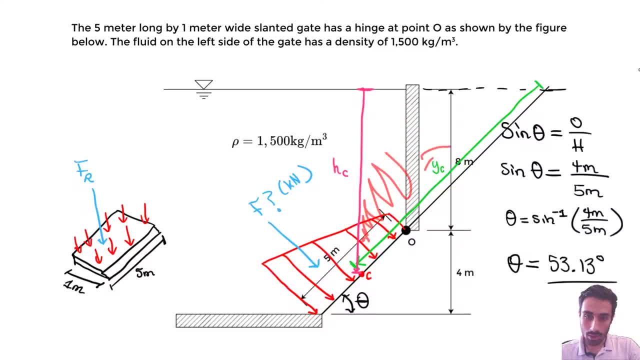 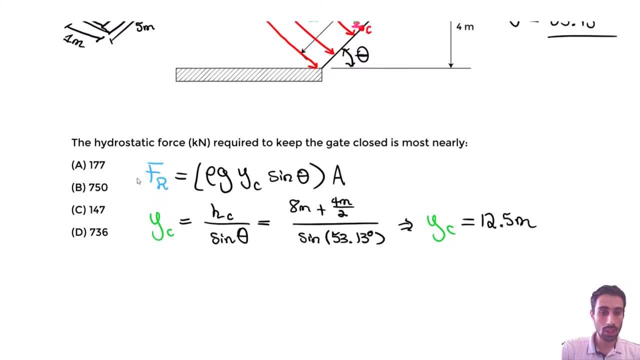 on right And we just found YC by doing SOHCAHTOA. We just found this, since we know HC, So that's where that comes from. We found YC. Finally, we can find the hydrostatic force, Because we have YC and we have the 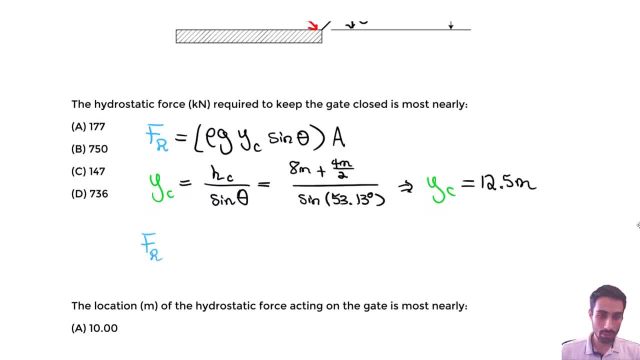 angle. we can find the area easily by doing base times height. So we know FR. We take the row, the density is 1500 kilogram per meter to the third. Then you multiply by 9.81 meter per second squared And you take YC, which is this 12.5.. 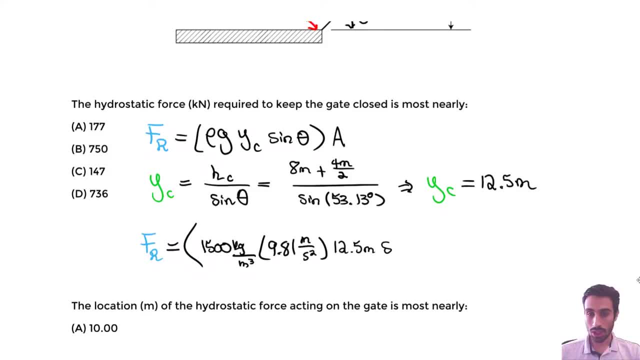 12.5 meters. Then you do sine of theta, So this is a S Sine of theta. We know theta is 53.13 degrees. Then, close parenthesis, all of this Multiply by the area, So the area is into the page right. You want to look at it from this view? So it's just base times. 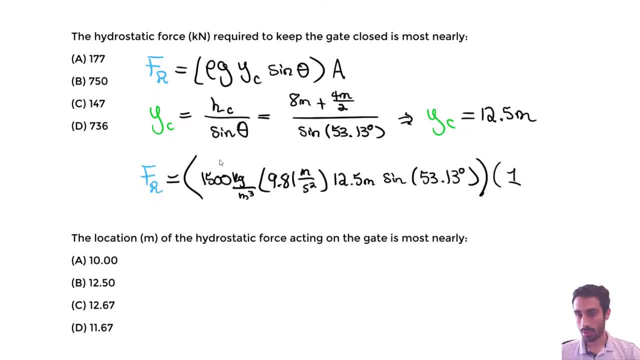 height 1 times 5 meters. So you take 1 meter times 5 meters, So then we can solve for the resultant force, And for that you should get about 736 kilonewtons. So here the output will be newtons. You divide by 1000 to get kilonewtons And we get approximately. 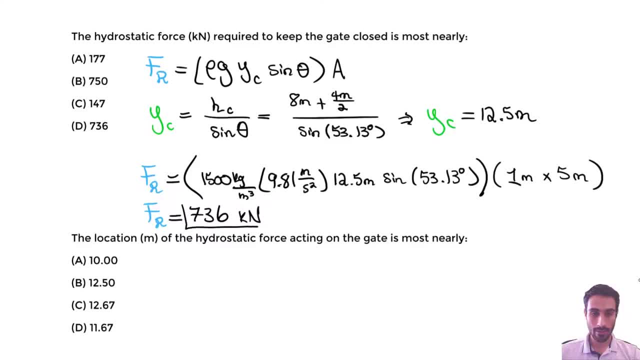 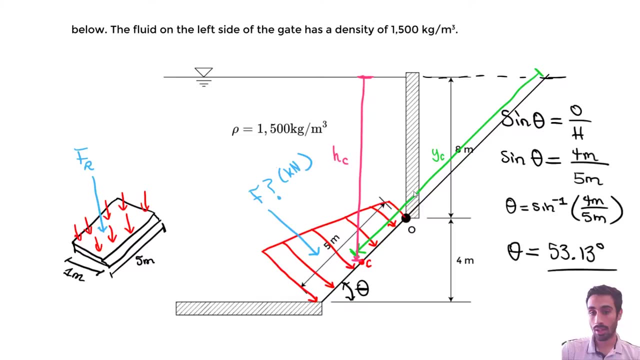 736 kilonewtons. So this is the answer for this portion 736.. Once again, I just used the equation in the handbook. I didn't want to complicate it here. I know some people can use they use volumes. You can take account for the volume and just add up all the volumes. 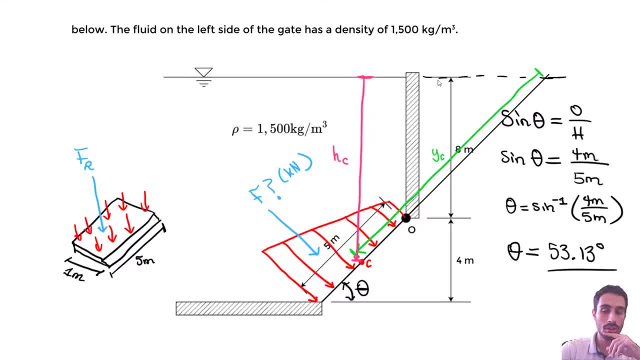 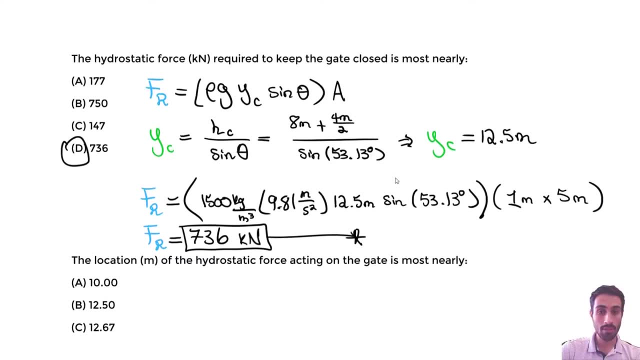 shapes of volumes. There's also other methods to solve this, But I want to make it simple and just use the equation in the handbook for slanted surfaces. So we have that, And the last step is the location of this hydrostatic force. So we 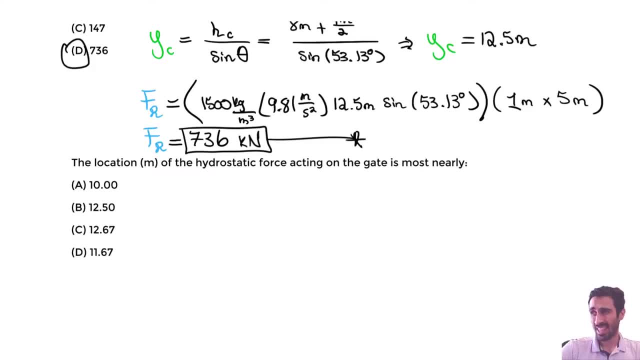 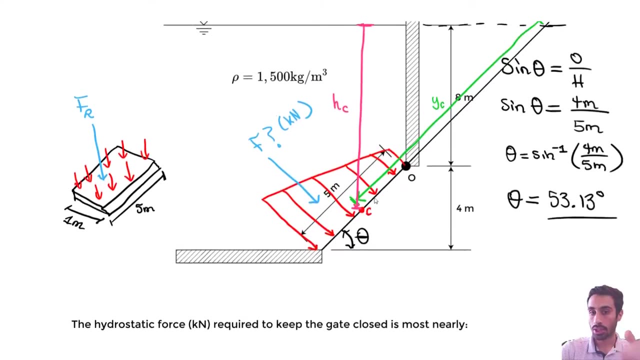 know, in the handbook, if you look at the figure carefully, it says that we have a centroid and we have a center of pressure. The force always acts at the center of pressure. It's slightly below the centroid. Always, The force always acts at the center of pressure. So 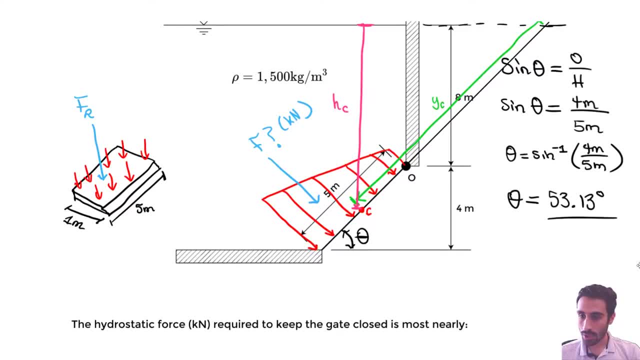 it doesn't act at the centroid, It acts somewhere here at the center of pressure, So let's call it Cp. It acts at the center of pressure. It's below the centroid And that's denoted in the figure in the handbook. 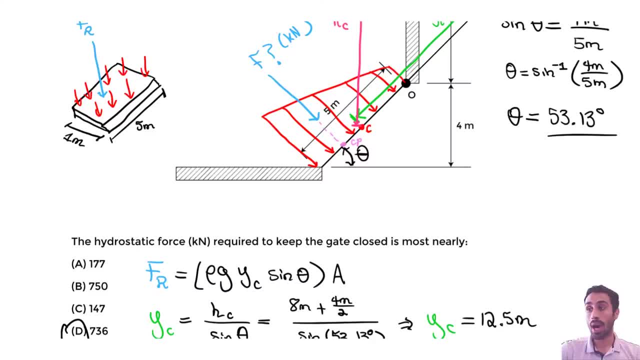 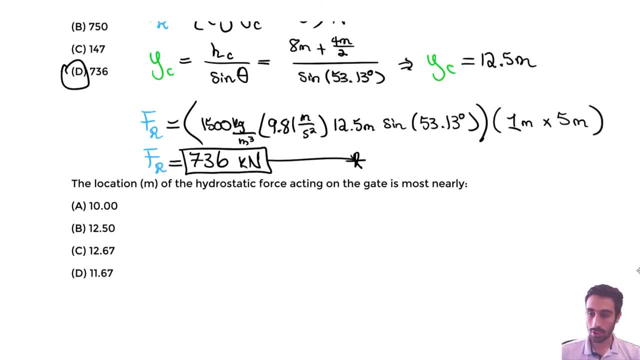 So let's find that distance And it's going to be Ycp. There's an equation for that in the handbook. So the equation is Ycp. the distance to the center of pressure is going to equal to the Yc which we did find in green right. Yc we have, Then we do plus the Ix. 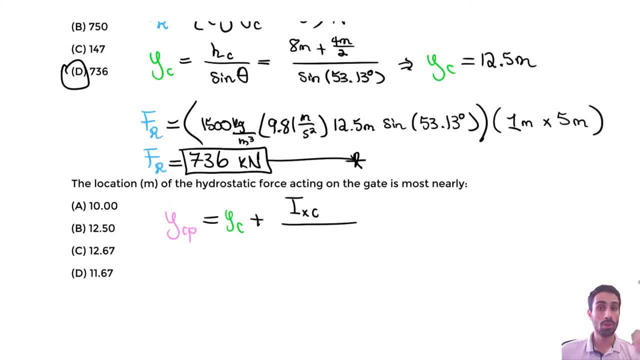 about the centroid. It's the moment of inertia about the centroid, For this basis, For this basic shape. Here it's just a rectangle, right, So that's going to be that. And then we take Yc on the bottom. Yc, this is the same as this. Then we multiply by the area. 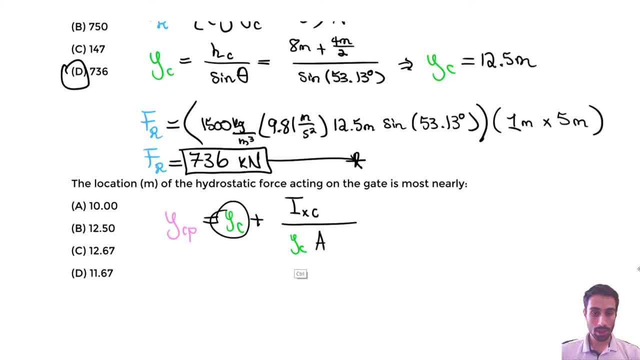 for that shape, the rectangle. So we know this, We know this, We solved it from the last question, And Ixc is going to be simply what? So you should know this For simple shapes, if you don't try to memorize this equation, 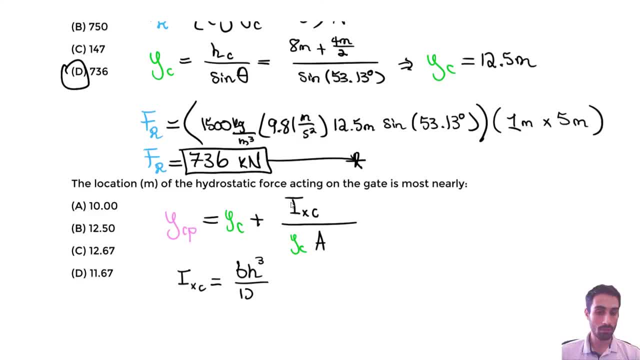 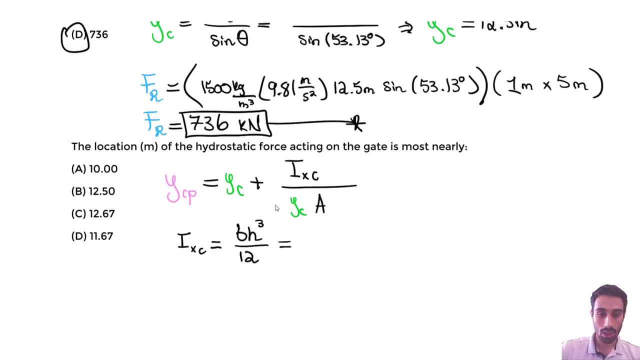 What you do is base times: height to the third divided by 12.. About the centroid, This is under the static section for those basic shapes. So in this case we take the base. What's the base? We know, based on, the width is 1 meter, The height is 5 meters. So we take 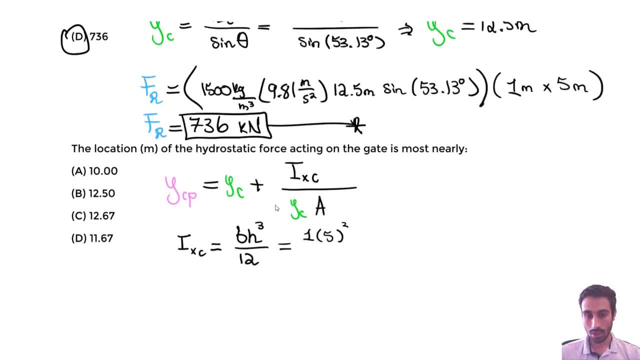 1 meter times 5 meters to the third, divided by 12.. Then we know Ix about the centroid, will give us about centroid, So it should be units. meter to the fourth And I got 10.42.. Meter to the fourth. So we. 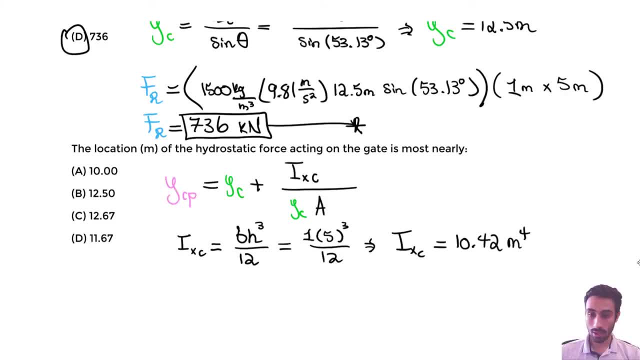 have that. All we do is plug it here and solve for Ycp that distance. Ycp equals. Yc. we said is 12.5, as we determined above, Plus We take this, which is this 10.42. Meter, to the fourth. It's the moment of inertia. 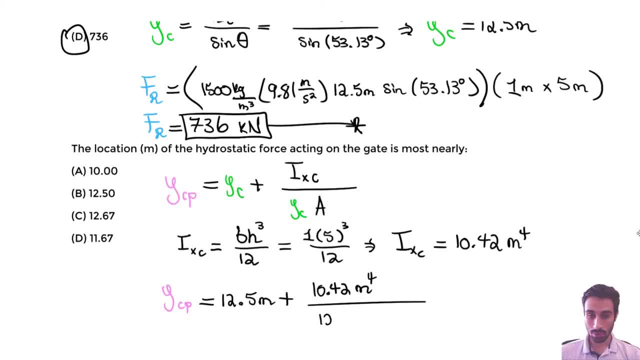 about the centroid. We take Yc, the same as this, 12.5 meters, And you multiply by the area. In this case it's just 1 meter times 5 meters. So then we can solve for that answer. 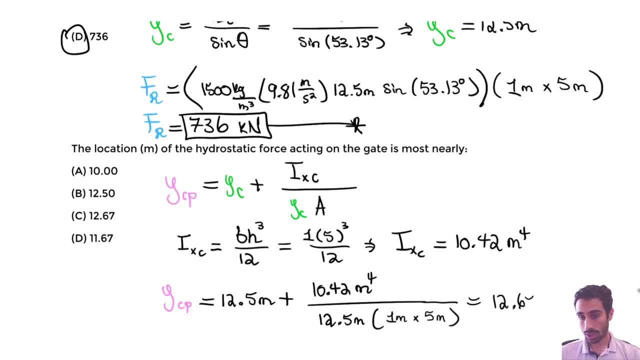 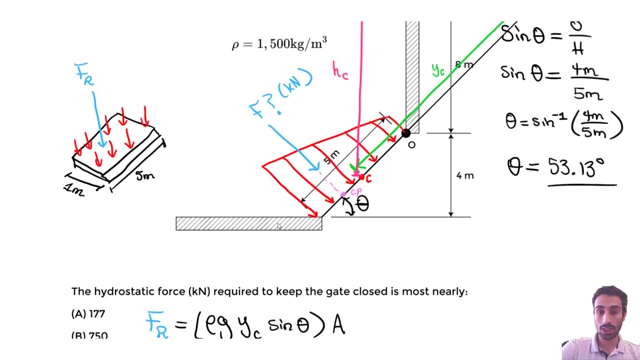 And we should get 12.67 meters. So this is the distance where this force actually acts, From that, that slanted distance from the top water surface. So it should be C And we can tell that this is below the Yc, because we said that Yc is 12.5.. This is slightly below that, right It's. 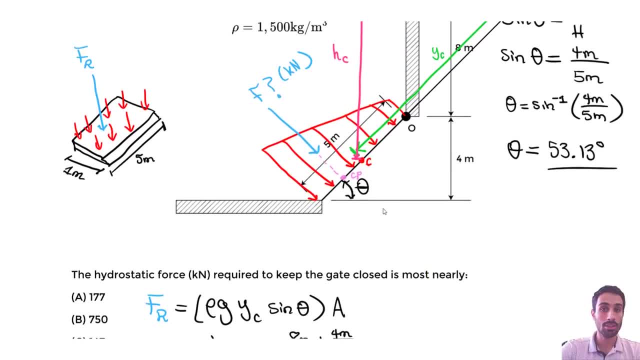 12.67.. So it makes sense. The final answer does make sense, And I think that's all for this video. Thank you.